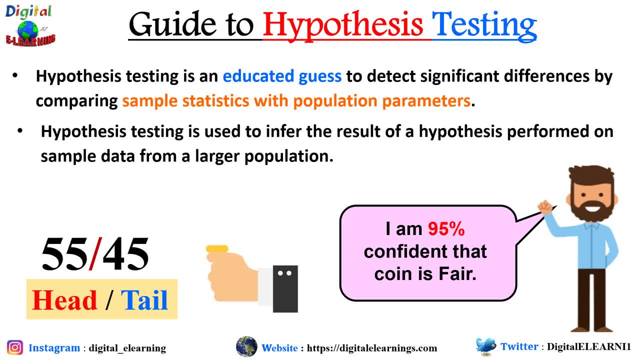 evidence to suggest that coin is unfair. come up with hypothesis that i am 95% confident that the coin is fair. but if we flip for rather 100 we get 75 head and 25 tail. can we still have that confidence? i am not sure, because in this case 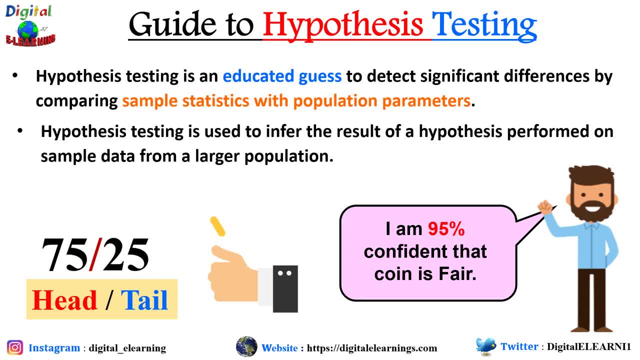 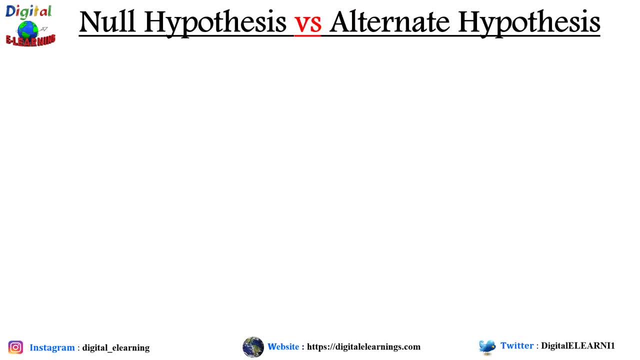 we cannot say the coin is still fair. the extreme low probability is the evidence that coin may not be fair in this case. so there are two types of hypothesis: null hypothesis and alternate hypothesis. let us understand each one of them one by one. we start with null hypothesis. it is denoted by 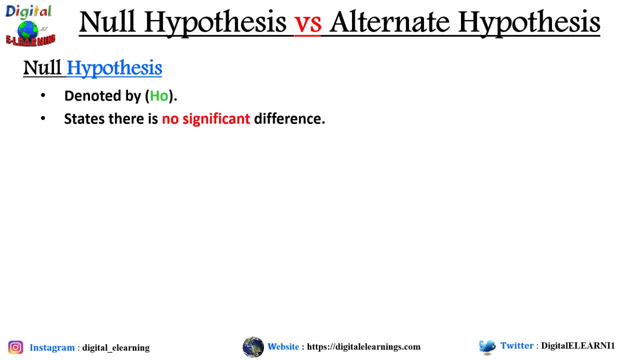 h naught. it always states that there is no significant difference and the difference that you have is just by random chance. it means that there is no significant difference between the population mean and the sample mean. it is always the accepted fact and is referred to as the status cube. it always contains the equal to sign and is 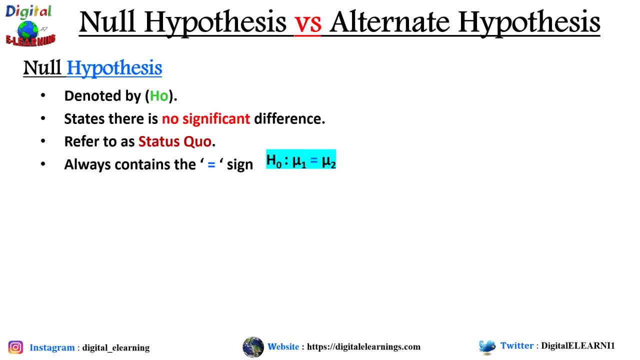 given by equation, as h naught equal to mu 1, will be equal to mu 2, that there is no difference between the two population parameters. if the difference between the sample statistics is large enough, assuming that h naught is true, then we have to reject h naught and conclude. 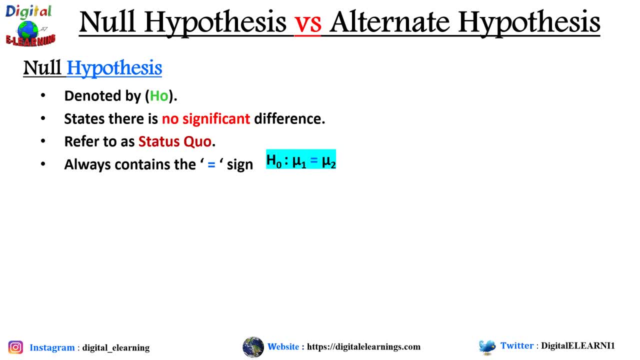 that there is a difference between the populations. now let us see what is alternate hypothesis. it is denoted by h a or h 1, which means there is a significant difference and the difference is caused by some non-random chance. h 1 will always contradict h, naught that is. 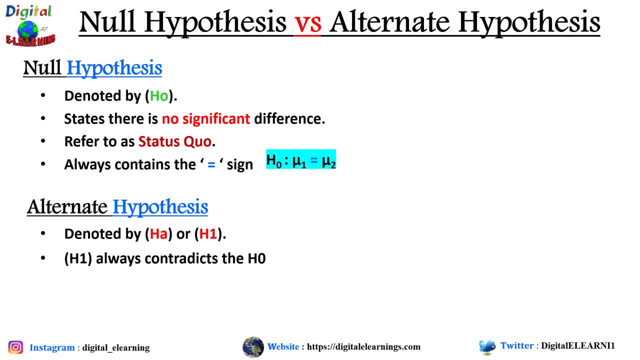 the null hypothesis alternate will always contradict the null hypothesis. alternate hypothesis is also known as the research hypothesis and they are influenced by some non-random cause. so if the null hypothesis is rejected then we will have to find out the evidence to support the research hypothesis. it always challenges the status q that is the null hypothesis. it never. 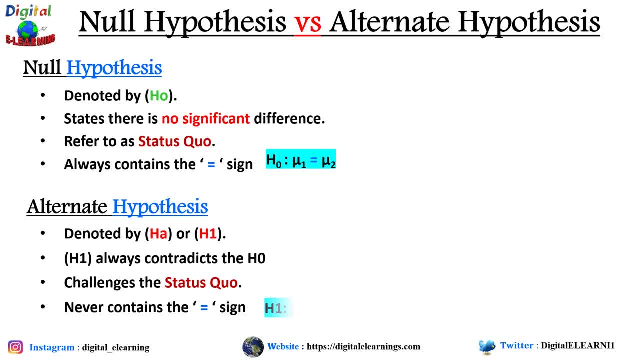 contains the equal to sign. so we have to find out the evidence to support the research hypothesis and we represent alternate hypothesis, as u1 is not equal to mu2. now, out of this null or alternate, only one can be true. there can never be a scenario where both. 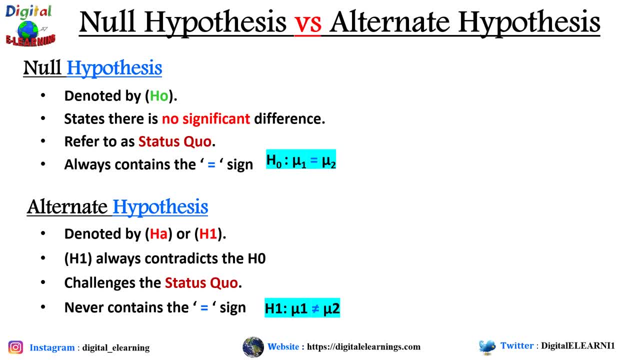 suggestions are true or both are false. either null is true or alternate is true. let's take the same case. we flip the coin. we get ideally 50 tails and 50 head out of 100 flipping. so our null hypothesis is that coin is fair. so we have p equal to 0.5. an alternate will be. 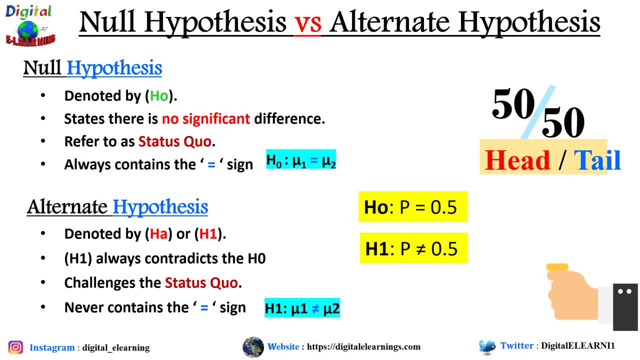 we challenge the null that it is not equal to 0.5. that means the coin is not fair. that means if we flip 100 times, we could get 70 head or 30 tail or 60 head or 40 tail. so that is how you frame your alternate hypothesis and null hypothesis. 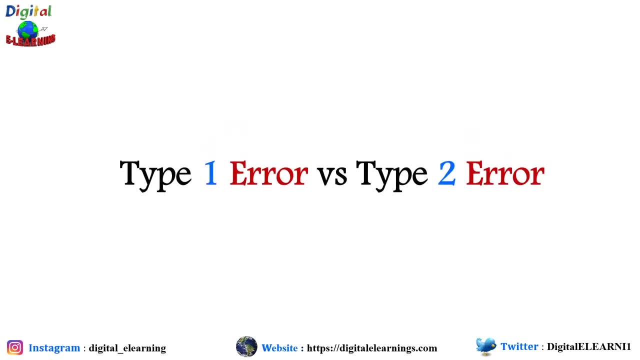 also, we have the tough regression response here. acceptedahl, the doubt table was always in order to distinguish till we get enough answer. now, making a statistical decision always involves some kind of risk, and this risk, in hypothesis testing, we classify in terms of type one error and type two error. to understand it a little more, let's look at thislikethis graphics: on the y-axis, we have the verdict in the form of whether the person should be jailed or set free. on the x-axis, we have the truth in the form of whether he is innocent or guilty. on the y-axis, we have the truth in the form of whether he is innocent or guilty. 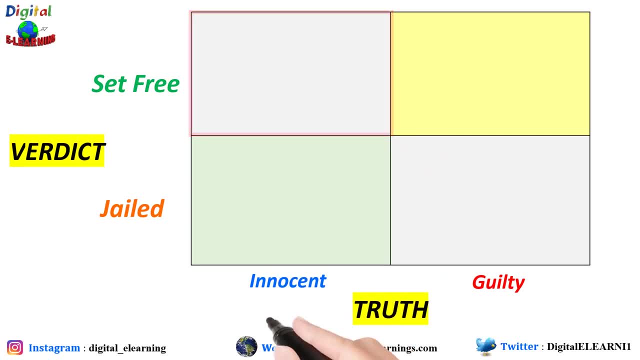 T. So if someone who is innocent should be set free, that is the correct decision. Now, if someone who is innocent who is jailed, that is not the correct decision. That is the type 1 error, or alpha error. We call it the level of significance, Also known as the false positive. 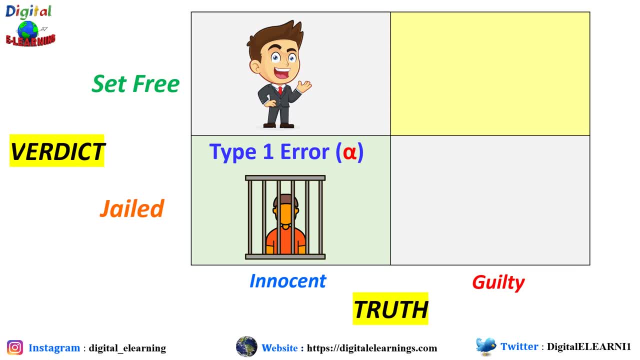 So if alpha, or the level of significance, is 5%, that means out of 100, every 5 would be awkward due to chance. Examples of type 1: error could be rejecting the good parts or the producer's risk, or jailing someone who is innocent. Now let us look at the other one, Someone who is guilty. 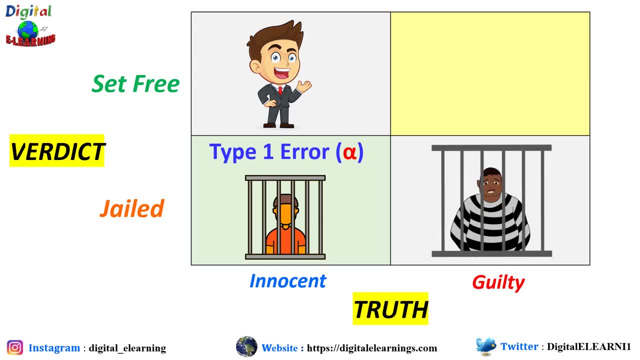 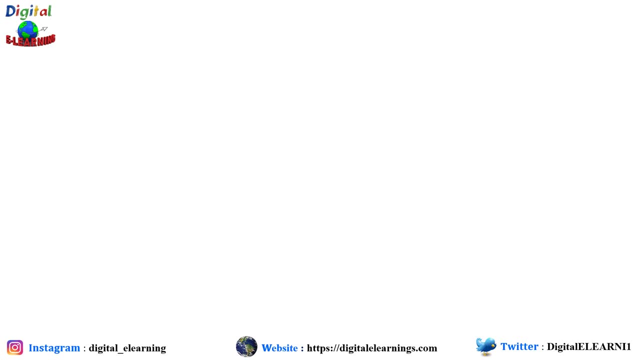 should be jailed. that is the correct decision. But someone who is guilty if you set that person free. that is not the correct error. That is we call it a type 2 error or beta error. We call this as false negative. That is, the error made by accepting or retaining a false null. 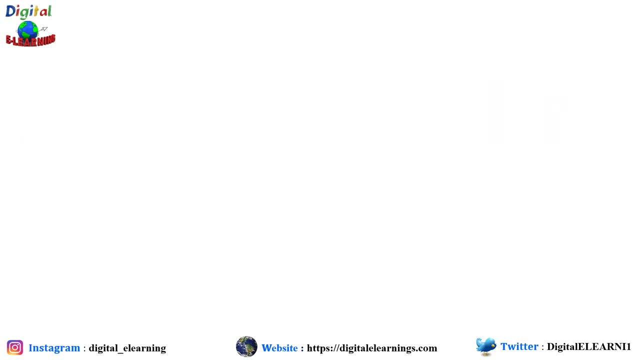 hypothesis. So example could be accepting bad parts or the consumer risk or setting someone who is culprit. The best example from the recent could be: the test result says that you have coronavirus or covid-19. But actually in real case it is not true. So that is the. 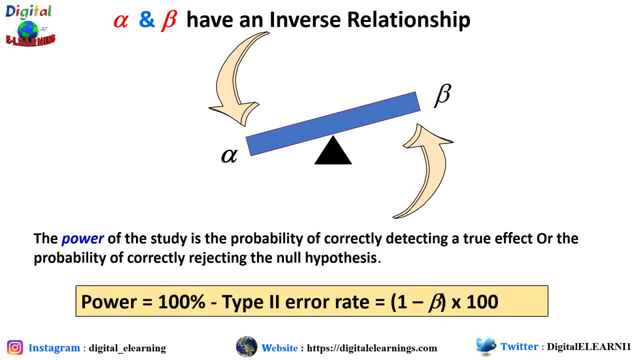 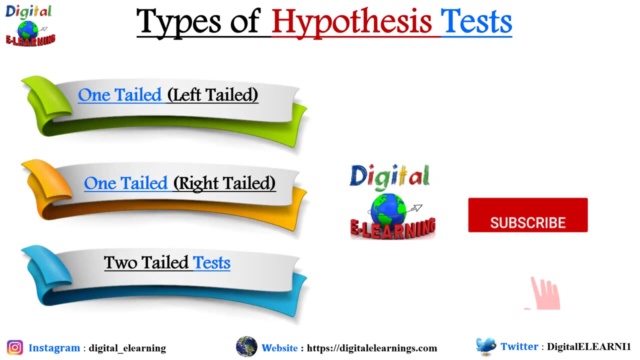 type 1 error. But in other case, if your test result says that you don't have covid-19 or coronavirus, but you actually do have, that is the type 2 error. This is the best example of type 1 and type 2 error In hypothesis testing. we need to judge whether it is a one-tailed test or a 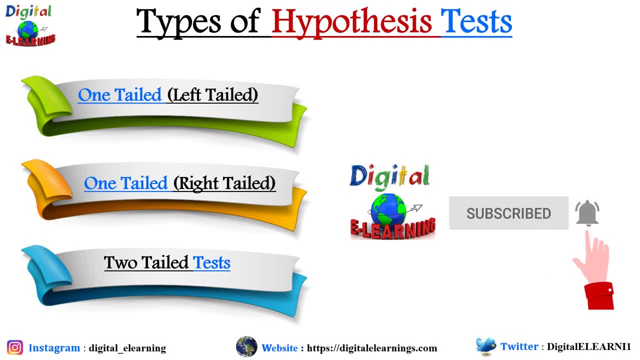 two-tailed test so that we can find the critical values from z-table or t-table, and then, by comparing these test statistics value with the critical value, we can come to conclusion whether to reject the null hypothesis or fail to reject the null hypothesis. So how can we tell? 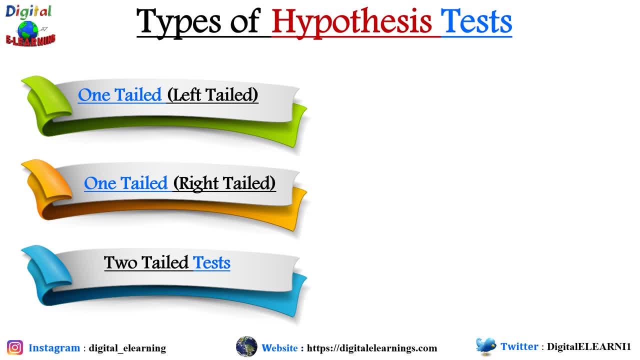 whether it is a one-tailed test or a two-tailed test. So it all depends upon the original claim in the question. So we look at each one of these one-tailed test- left-tailed or right-tailed- and two-tailed test in a little bit more detail. So what does you understand by one-tailed test? 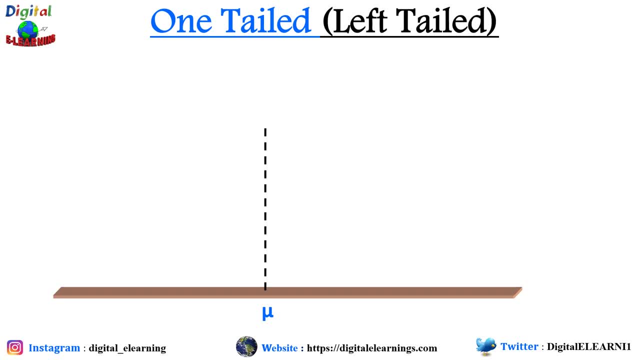 or left-tailed test. So before that, let us understand what do you mean by tail. So tail in hypothesis testing refers to as a tail at the end of the distribution curve. So if it is on the left side it is a left-tailed test, and if it is on the right side it is a right-tailed test. So in this, 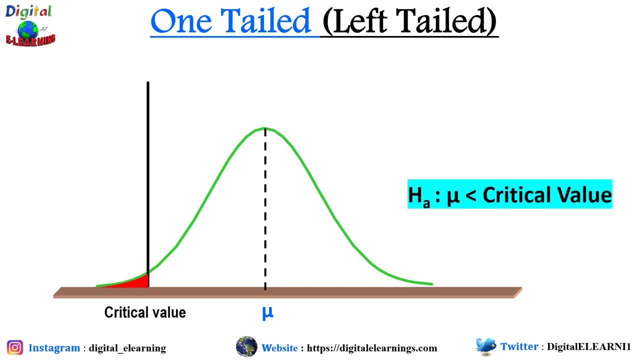 case: left-tailed test. this is my rejection area, marked as red. So we call it with the alpha level of significance. So if it is on the right side it is a left-tailed test and if it is on the right side it is a right-tailed test. Suppose the null hypothesis state that mean is greater than or.